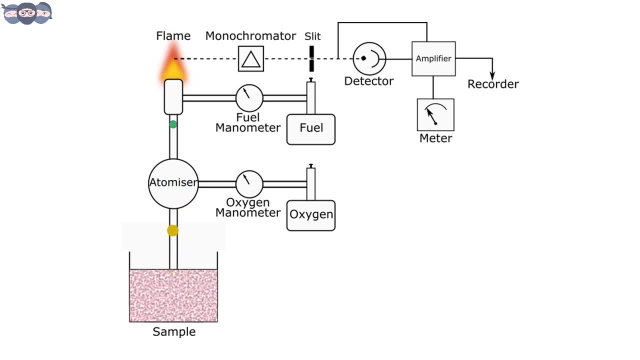 some kind of oxygen and fuel. This is obviously a kind of fuel, but that can be used as an cumulus. The atomizer can also be used as an action device. If the instrument is placed near the Haggard Converter, converts the sample to aerosol and passes this aerosolized sample to the next. 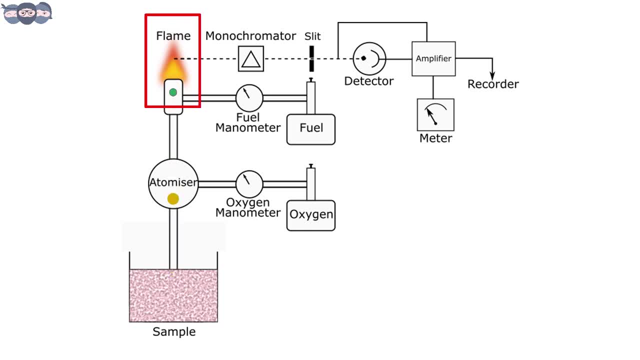 unit. The next component is the flame. The flame is employed to heat the aerosolized sample and provide energy to the atoms present in the sample. The atoms take up this energy and go to higher atomic state. The flame is followed by a monochromator which filters out the wavelengths and the final 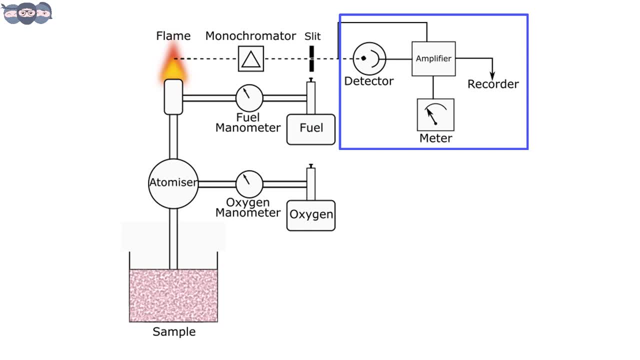 part of the instrument is the detector and display. Now let us understand the working of this unit. As stated earlier, the sample is first converted into aerosol form, Then this aerosol is made to pass into the flame. The aerosol contains the atoms from the sample. 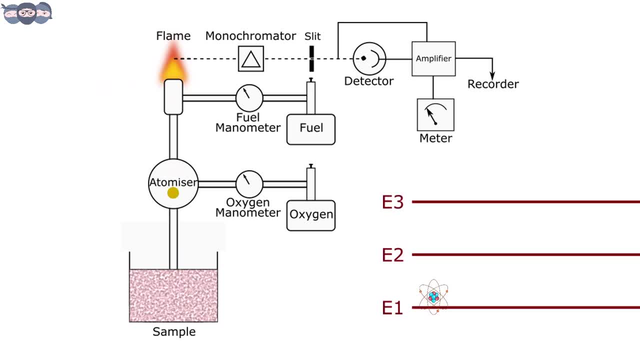 Once in the flame, these atoms absorb energy. The energy differences between the atomic states is different for different atoms. As a result, different atoms will absorb different amounts of energy, as required by them. These atoms cannot remain in the higher energy state for too long. 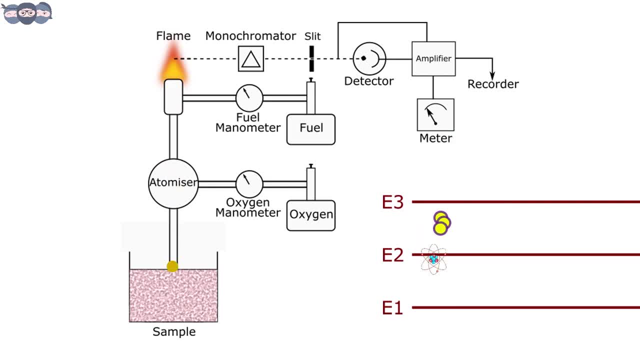 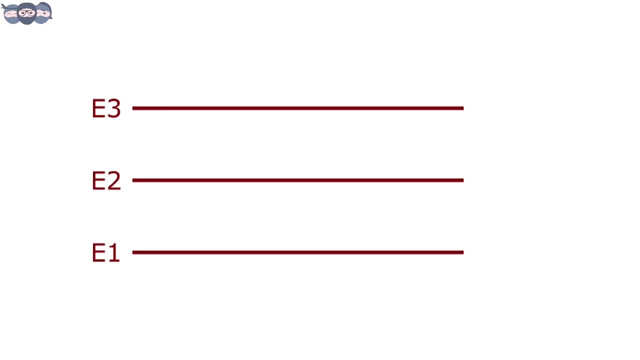 As a result, they fall back to their original atomic state by releasing energy. The energy is released in the form of photons. These are atomic emissions. The analysis is performed. However, the same reaction is achieved by studying these atomic emmissions. As discussed earlier, the different atoms will have different energy levels. 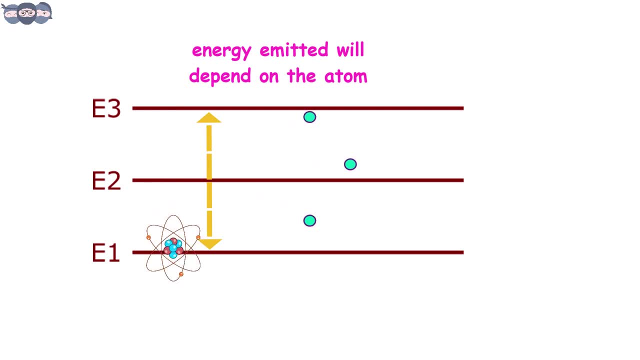 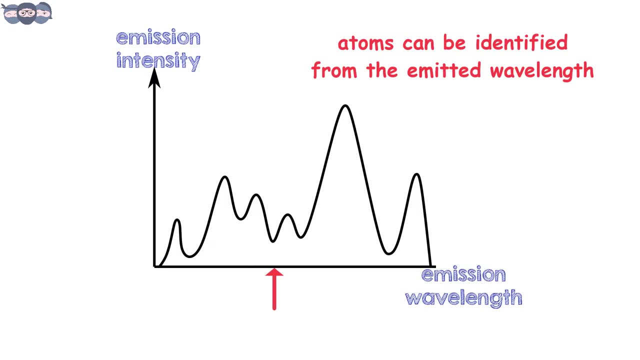 Hence the energy emitted by atoms will also be different. for different atoms, The emotions will have different wavelengths. From this wavelength the experimenter is able to identify the type of atoms, Similarly the intensity of the emissions. This dependent quantity of the atoms present in the sample. If more the number of atoms, more is the intensity. 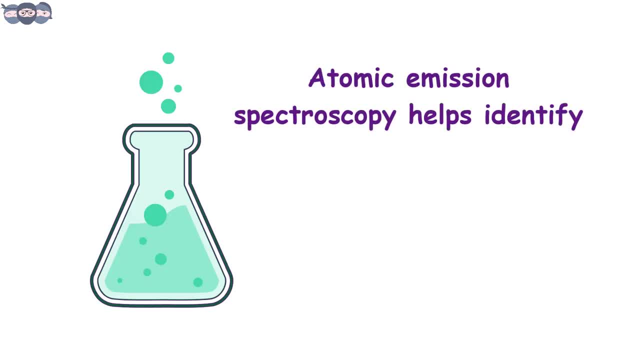 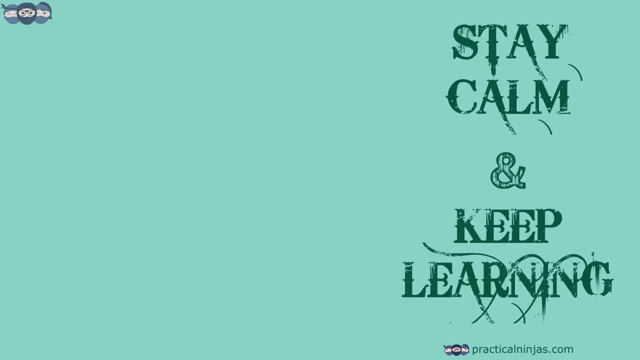 and vice versa. In this manner, one can identify a particular atom present in the sample as well as its concentration. Hit that like button and share the video with your friends if you have enjoyed it. Until next time, stay calm and keep learning. Peace out.